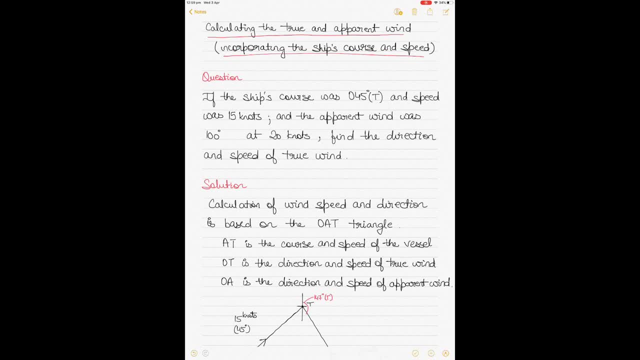 is, of course, the true wind and direction and the apparent wind is the resultant wind based on the ships course and speed. so that's the difference. so the question, and go straight into the question now. the question says that ship course and was 0 for 5 degrees true, and the speed of the vessel was 15 knots. the apparent wind was 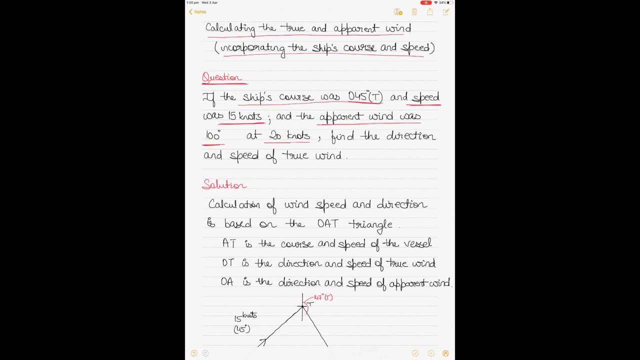 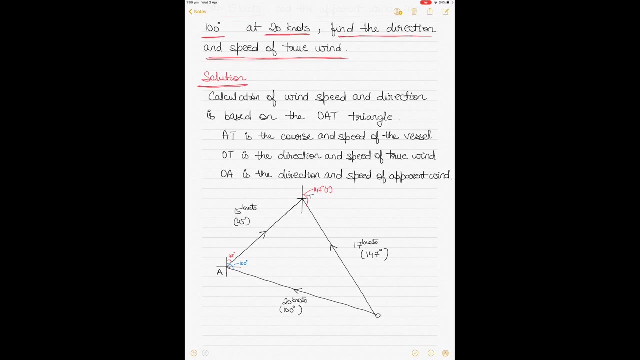 100 degrees, or direction of 100 degrees at 20 knots. what you have to find is the direction and speed of the true wind. all right, so before you go into this question, the solution, just remember that the calculation of wind speed and direction, which incorporates the ship's course, 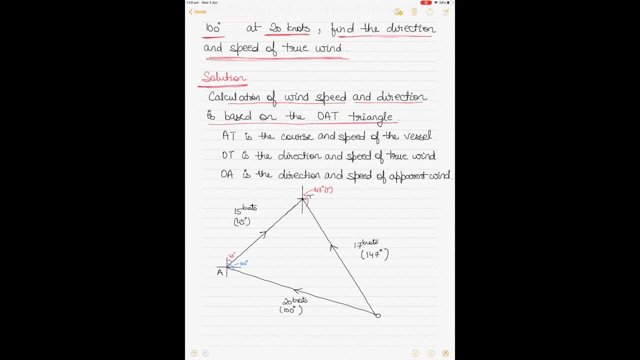 and speed is based on the o 80 triangle, so the triangle is o 80 and that's what we call it. all right, if somebody else calls it something else, it's fine, but it's the o 80 triangle in o 80 and I'll change the pin here. 80 is this ship's course and speed. all right, course and speed of the vessel. 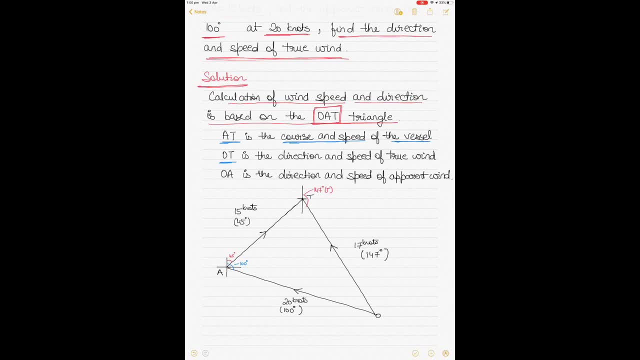 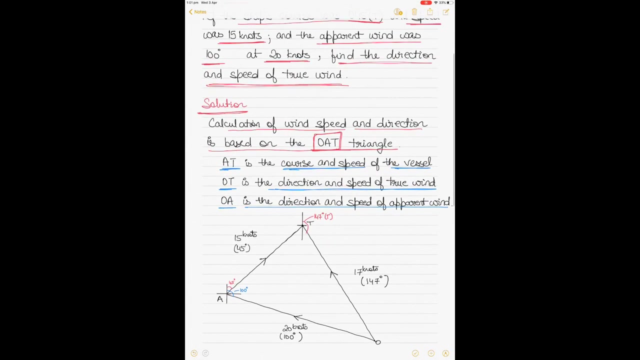 you, o, t is the direction and speed of the true wind. so here t stands for true and o, a is the direction and speed of the apparent wind, and this a will be apparent. all right, I've drawn the diagram for you here, but I'll show you how I drew it, all right. so, basically, these are the three. things are the three? 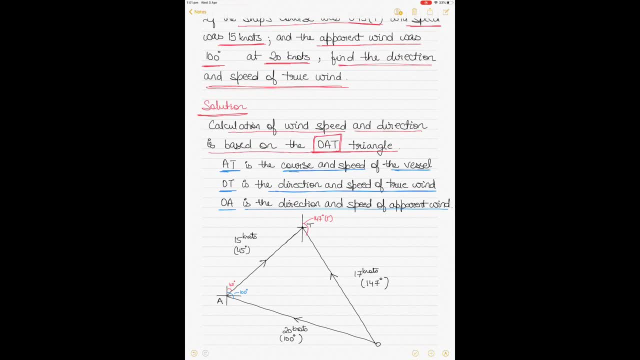 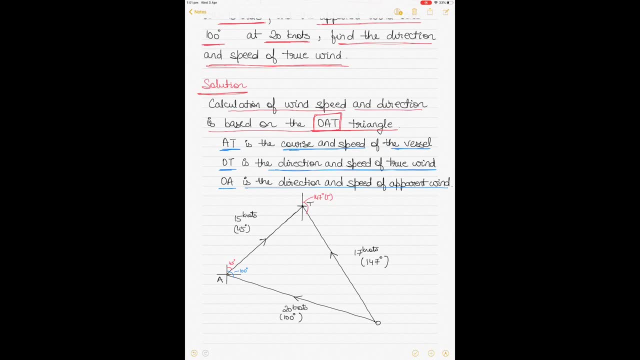 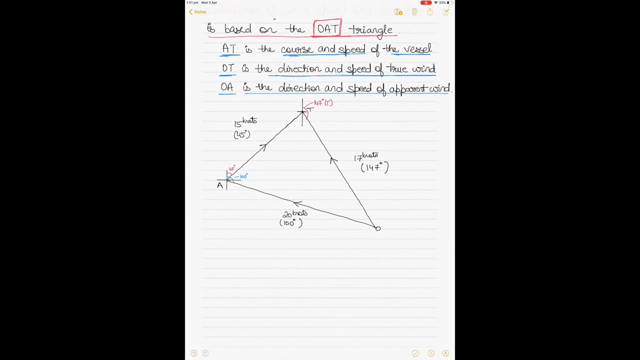 sides of a triangle you have to draw. you should be able to draw two sides and then you can calculate the third side. it's very simple. all right. as long as you get the direction right and the speed right, you should be able to calculate the third side. all right. so remember normally these o 80 triangles. 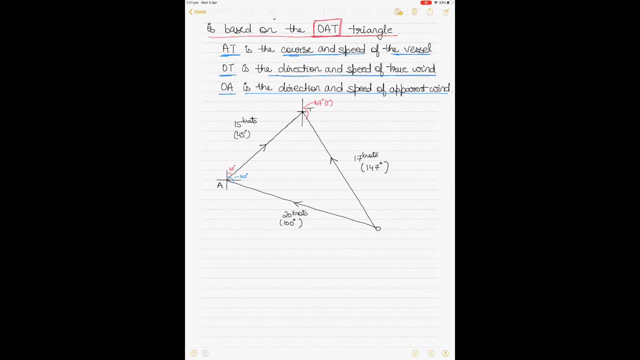 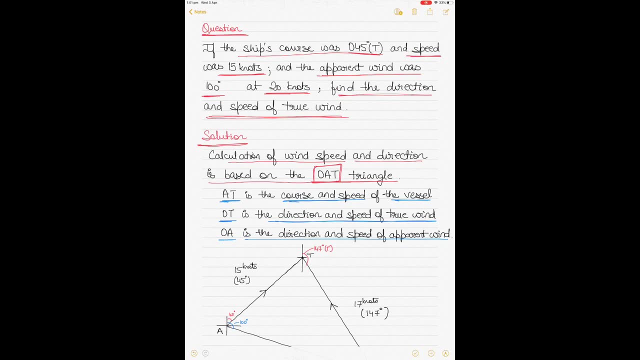 is drawn for one hour. it's a vector of one hour. so basically that means is if the ship is doing normally sometimes some questions, they intentionally make you draw triangles of two hours or more, normally one to two hours, but normally in these triangles you are going to stick to a vector of one hour. that means that if the ship speed was 15 knots you will. 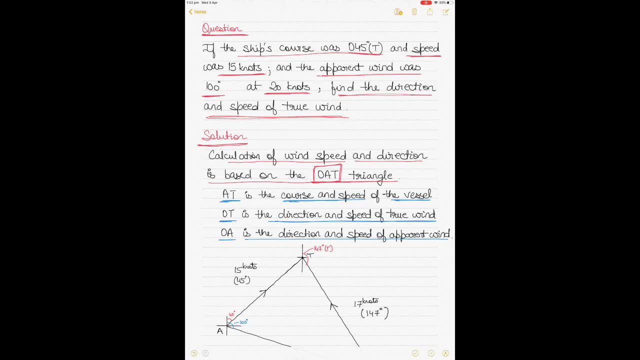 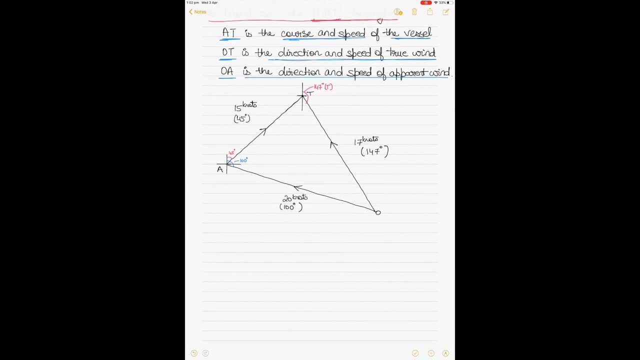 consider the ship's speed for one hour, which is 15 nautical miles, all right, and similarly the wind will also be taken, as for one hour only. so normally I will write it down here: it's a one hour vector drawing, one hour vector drawing. so you consider everything for one hour only, all right, sometimes. 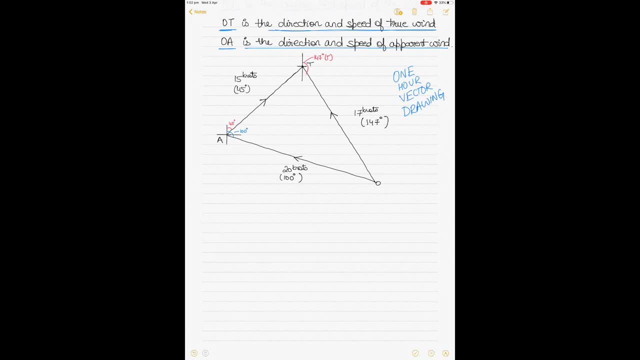 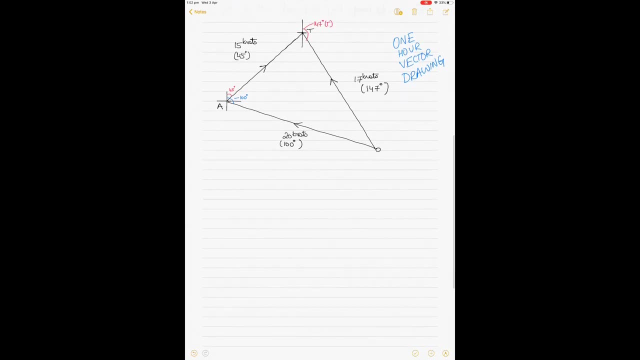 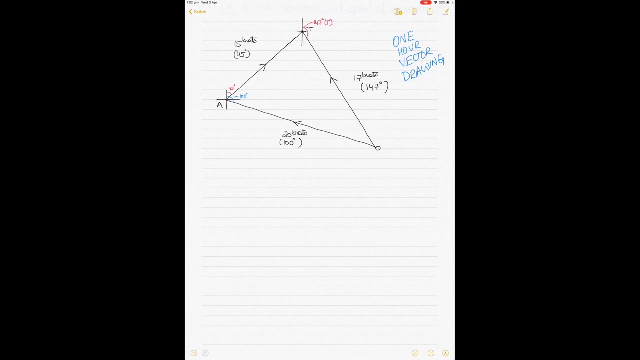 it depends on the question how they frame it. some some- sometimes some people- try to trick you into making triangles of more than one hour, but that's fine, all right, so I'll continue over there. so what you basically do is you start off somewhere, say because you know. 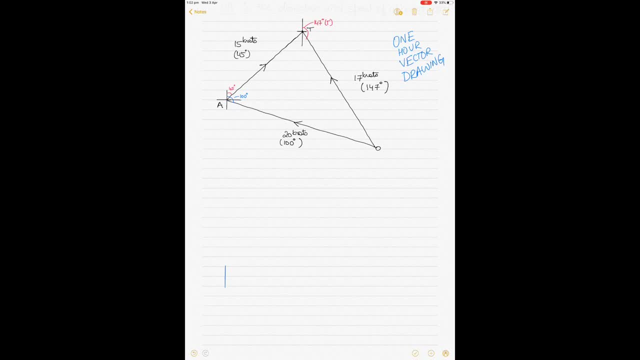 I am the idea. so you can start off somewhere. you can start off from the center of the page so say, for example, you draw a cross here, okay. so though, you just see what is given to you. so what is given to you is the ship's course and speed. so 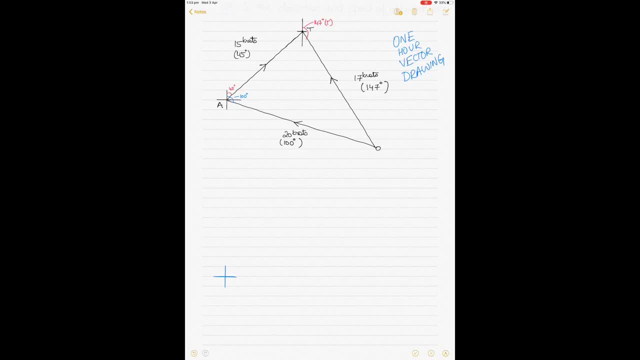 you can do is always draw that first. so ship's course and speed is signified by 80. so that basically means measuring from a going towards t. that's your ship's course. so just go in a direction of 045, because that's your true course. so measure 045 and draw a line and then take a. 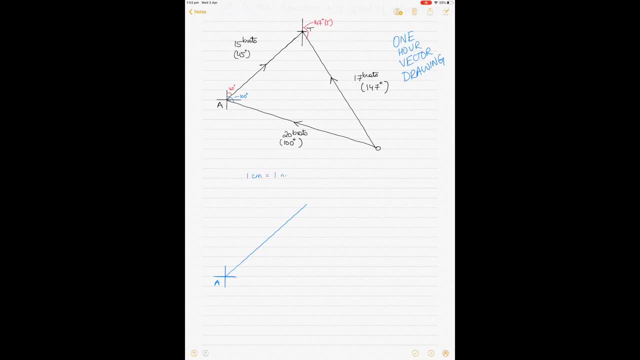 scale of, say, one centimeter equals one nautical mile. so your ship's speed was 15 nautical miles. ship's speed: 15 nautical miles in one hour, all right. so you draw 15 centimeters, you measure 15 centimeters, so we'll make this 15 centimeters, all right, in a direction of 045 degrees. and this: 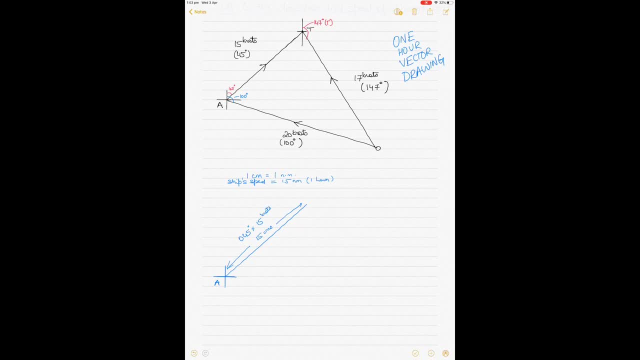 will signify 15 knots of speed in one hour. okay, then you stop here. then what you do is: the second thing you want you in the question is the apparent wind direction and again I said OA is the apparent wind. that means you have to measure from O going towards. 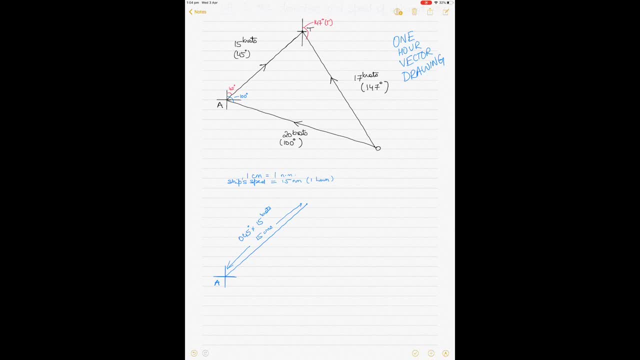 a that should be hundred degrees, so you have to go hundred degrees. so if this is, say, both north and this is East, signifying this is south and this is West, hundred degrees, so the east is zero, nine zero, so you go somewhere around here. so hundred degrees, you just go hundred degrees. 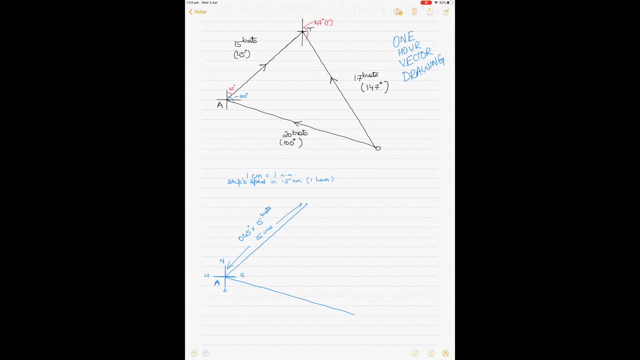 here, okay. and then, because the apparent speed is 20, measure 20 centimeters on the scale here. all right, keep going in. measure 20 centimeters. this will be longer than 15 centimeters, of course. so what I will do is I'll draw a longer line, straight line, all right. so this should be 20. 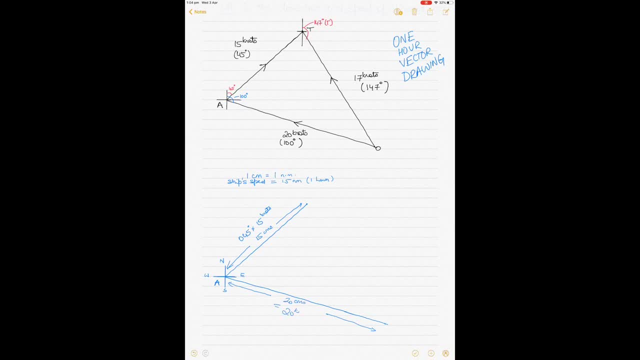 centimeters, which signify this is 20 knots or 20 nautical miles. so this should be 20 centimeters, which signify this is 20 knots or 20 nautical miles. so this should be 20 centimeters, which signify this, the nautical miles in one hour. that's what it signifies. all right, and the direction is of 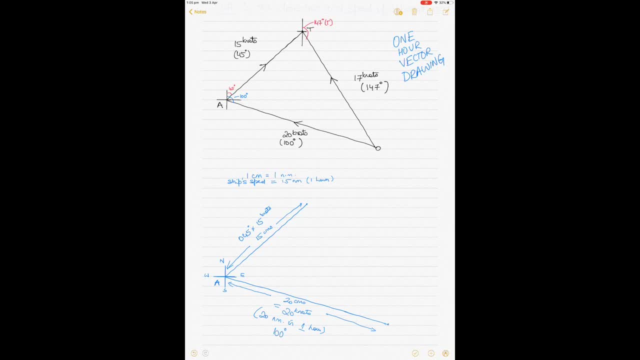 course hundred degrees, which is measured from O. so if this is O, hundred degrees, so because East is zero, nine zero, this is hundred degrees here. right then, all you have to do is basically connect O to T. this point here, where you do your ship's course and speed, this becomes T here, right? 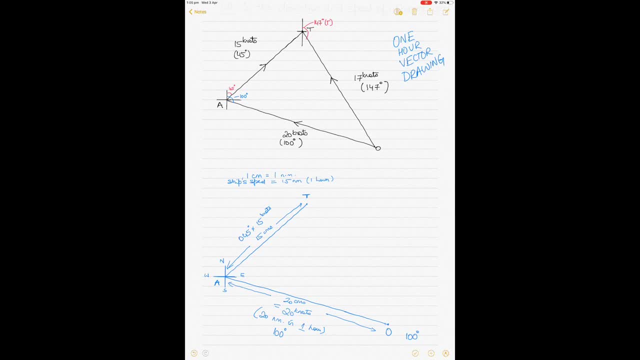 so all you have to do is basically connect O to T and remember that your true wind is also measured from O to T, so where your O will determine, the direction of O will determine what is your true wind direction, just like your apparent wind direction. all right, all then you have to do is 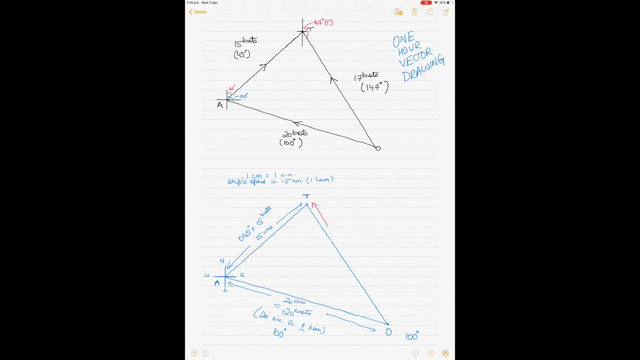 basically measure this distance here. all right, just measure this distance. this should be about 17 centimeters, which will signify 17 nautical miles. that means your wind speed, or true wind speed, was doing 17 knots in one hour. that's why your true wind speed will be 17 knots and the direction you can calculate by making 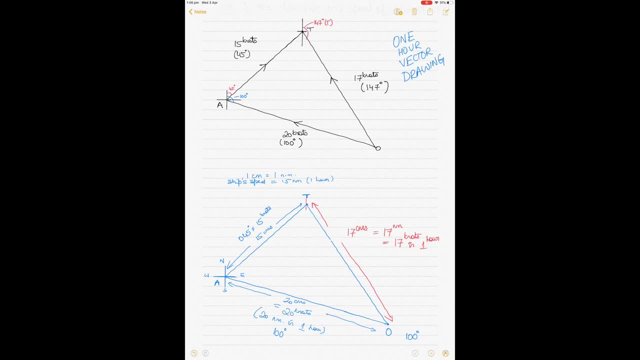 another plus here or another cross here, because you have to measure in which direction O is. so to measure direction of O, just measure from here to here. this should be about one, four, seven degrees, all right. so always measure going towards O. so although the direction of the true wind is measured,